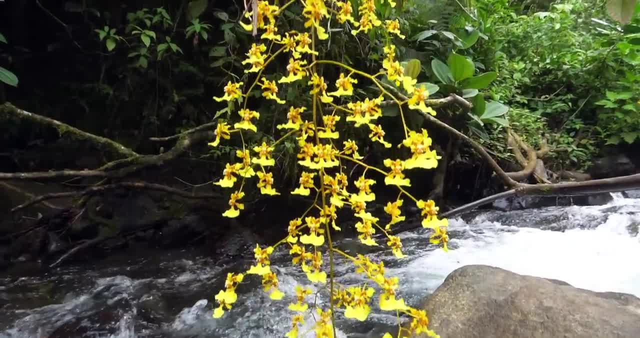 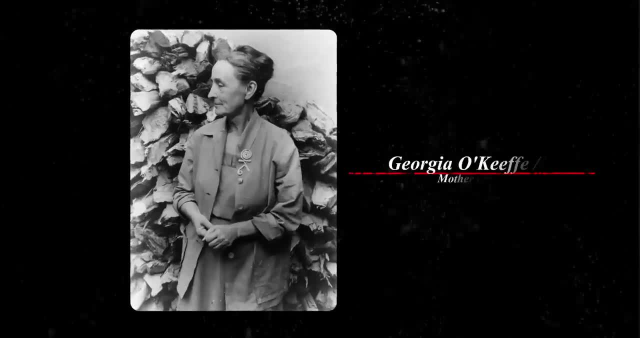 and have conquered almost every type of ecosystem. These seductive, deciduous herbs have been making people frisky for thousands of years. Great artists like Georgia O'Keeffe have explored their feminine beauty and likened them to some female body parts. 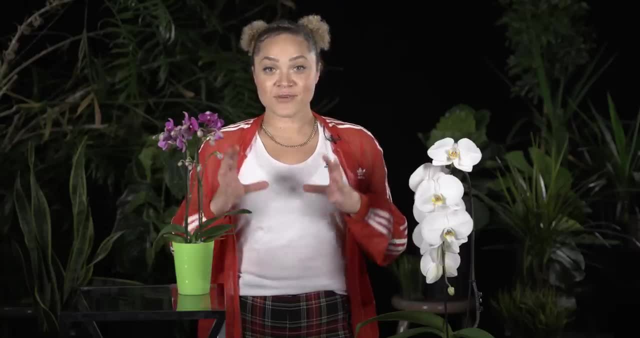 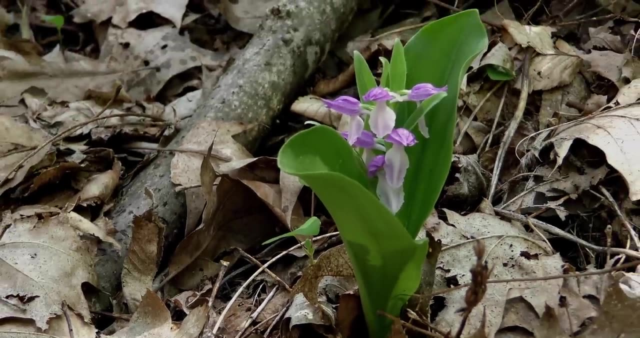 Even their name comes from the Greek word for testicle, due to the shape of their pseudobulbs, which were once even thought to be a foolproof aphrodisiac. Part of their success comes from being able to extract energy from the fungi that grows around its roots. 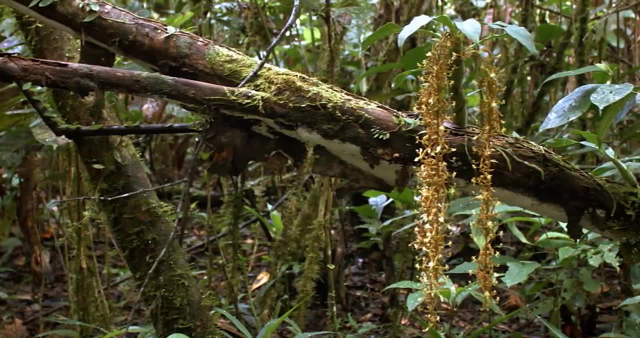 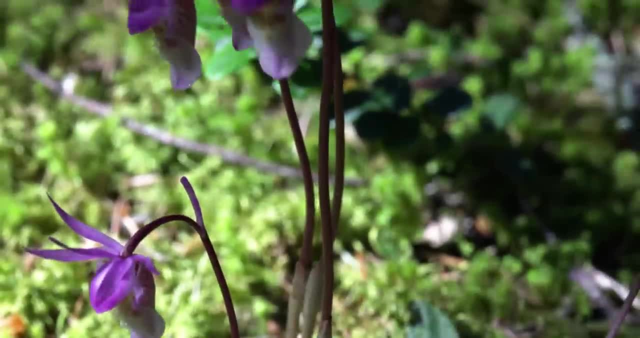 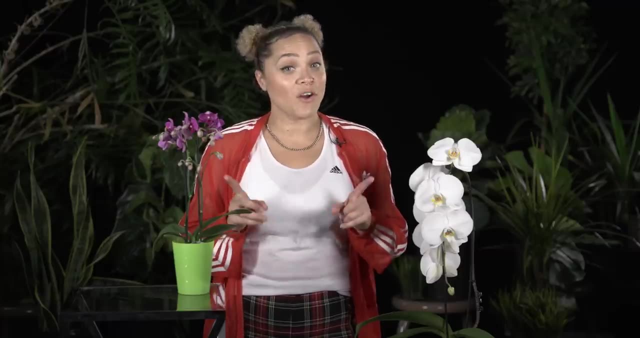 This has helped them thrive in low-light areas like in dense forests. Over time, this has led to a reduced photosynthetic capacity, meaning that several species can't grow without their mutualist fungi. They've also increased their chances of success by colonizing trees. 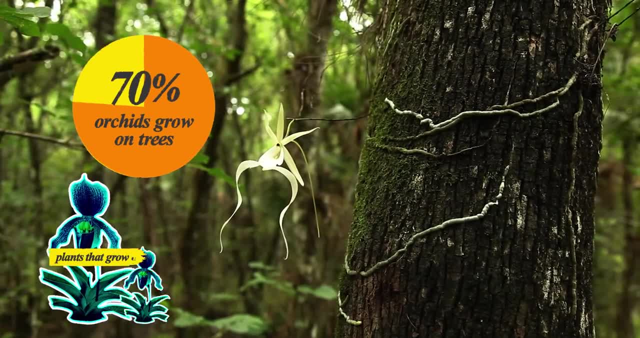 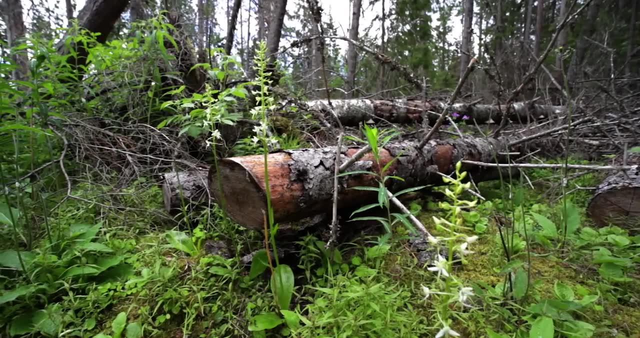 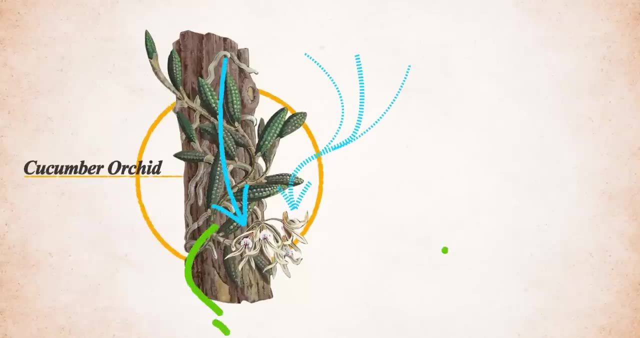 Seventy percent of all orchids grow on trees and two-thirds of all living plants that make trees their home are orchids. These species are amazing at absorbing nutrients from debris that accumulates on the tree. They also capture moisture from the air and tree bark and store it in their pseudobulb. 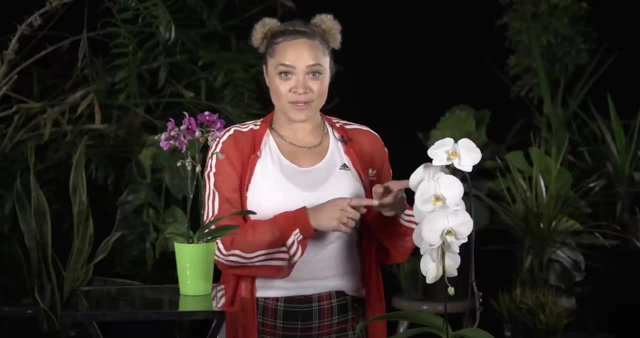 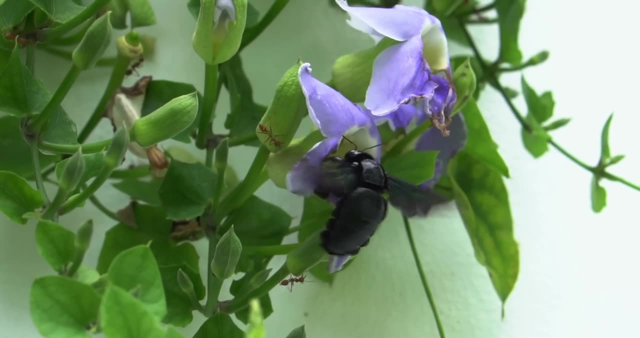 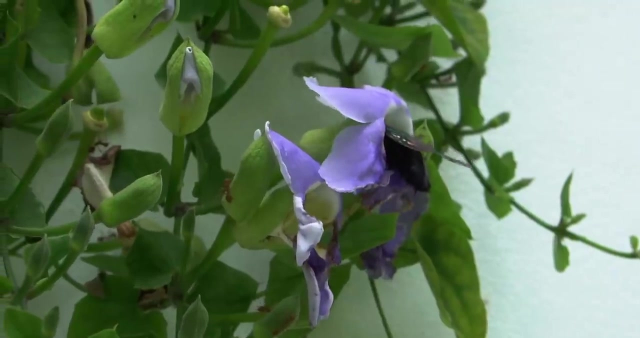 But by far their greatest tool is their flowers. They are absolutely stunning and incredibly good at tricking animals into pollinating them. Most flowers offer nectar as an incentive for insects to fly in and get covered in pollen, But about a third of orchids have figured out. 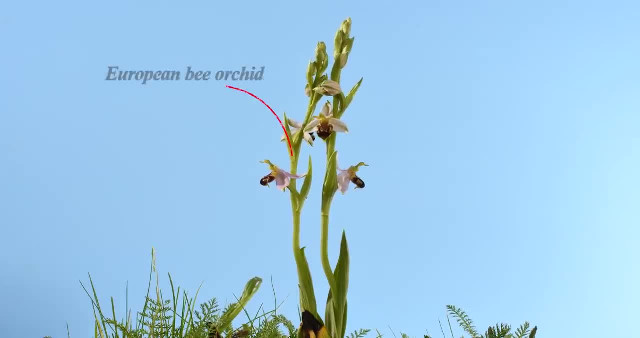 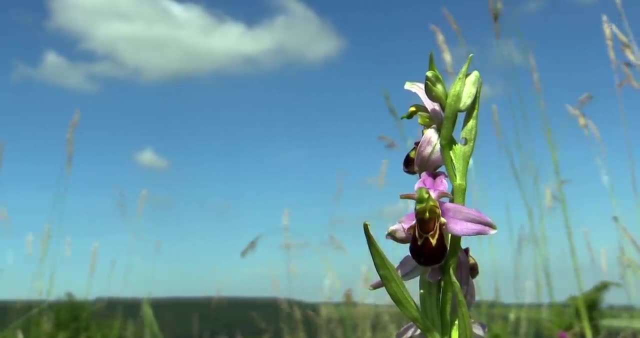 that a little trickery goes a long way. The European bee orchid is one of the best examples of this. Their flowers emit the sex pheromones of female pollinator bees. Males are attracted to them and are invariably duped into landing on the flower's labellum. 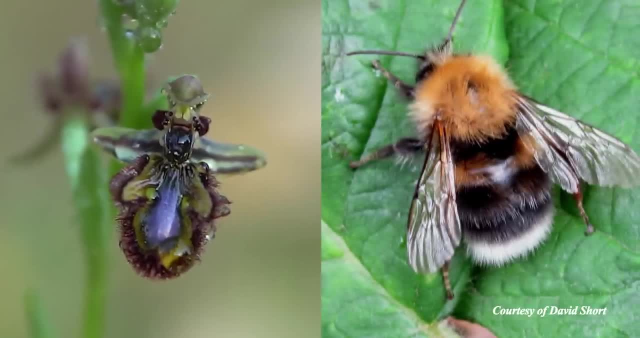 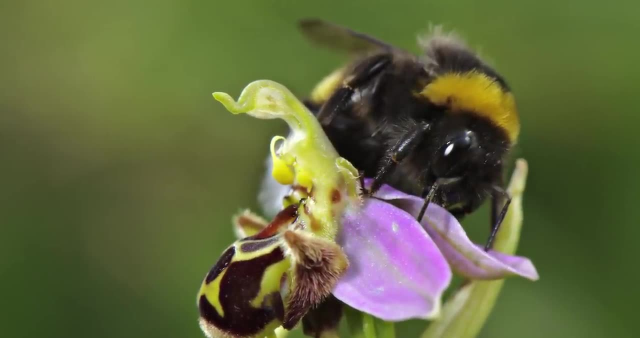 which is the same shape and color as the female bee. The males try to mate with the flower, thinking it's a bee, And in the struggle they get covered in pollen. After a while the male gets frustrated and leaves. He learns his lesson and stops visiting flowers with that scent. 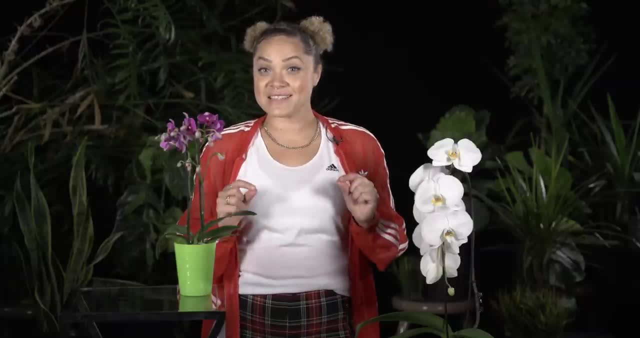 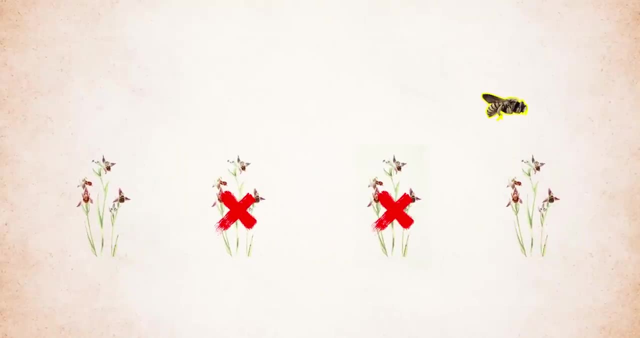 The brilliance of the bee orchids is that they emit slightly different bee sex pheromones, So the male will fly away and eventually get tricked again, this time by a different bee orchid. This ensures that the pollen doesn't go to a nearby bee orchid and prevents inbreeding.